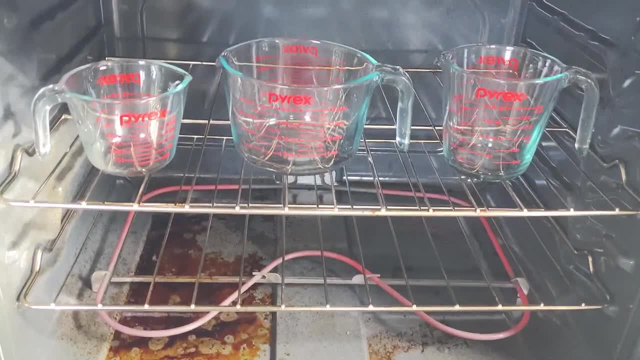 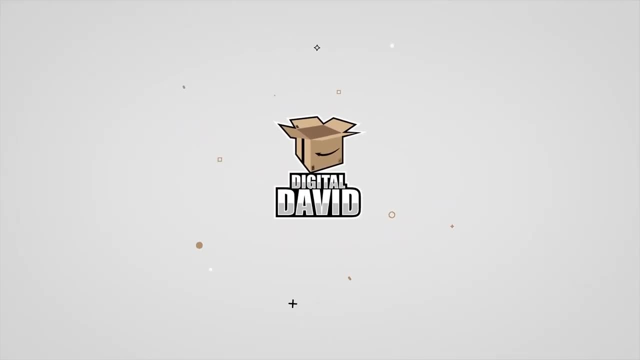 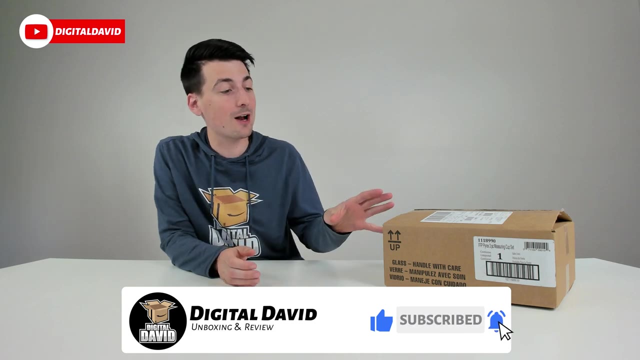 Here's your five minute checkup. So they've been in the oven for five minutes and you can see they look great. Hey everyone, Digital David here Today in this video I'm going to be checking out the Pyrex three-piece glass measuring cup set. I did purchase this product myself and any opinion 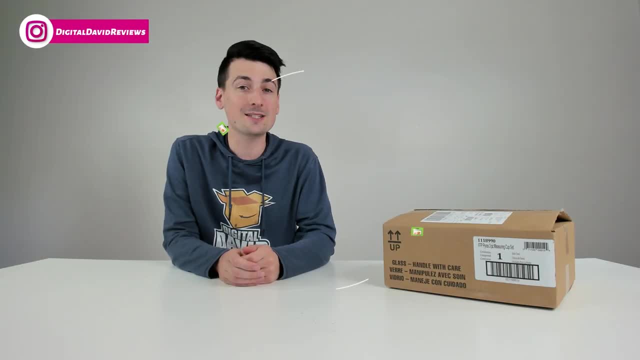 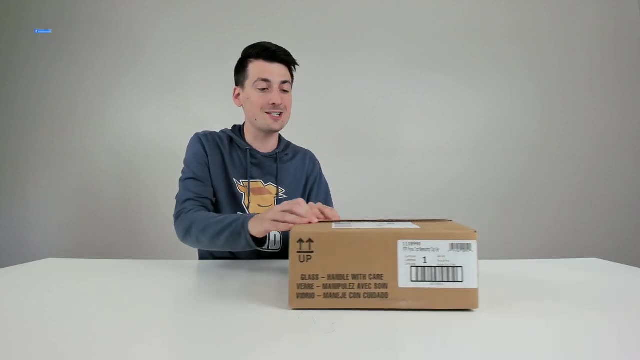 expressed in this video is strictly my own. That being said, if you're interested in this product, you want to find out more about it. the link to it will be in the video description. You can see the very simple product packaging. It ships directly in a non-discrete box right here. 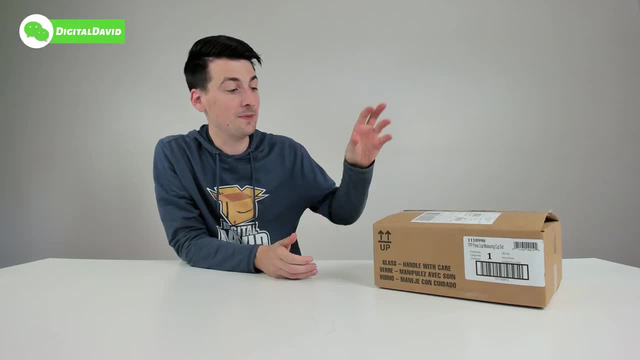 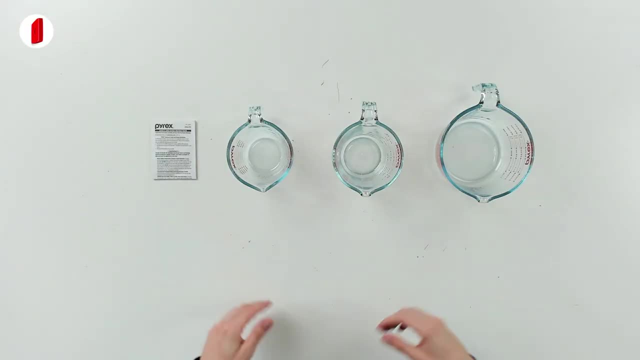 and as soon as you open it up, there's not another retail box, It's just the pieces from our set wrapped in there. So now let's go ahead. let's look at the contents. Here are all the package contents. First up, you can see we have our safety and usage instructions, followed by our three 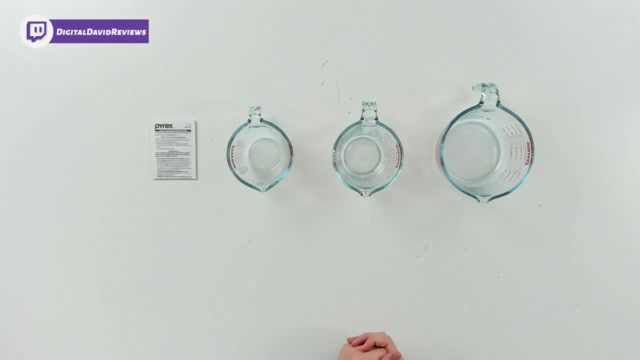 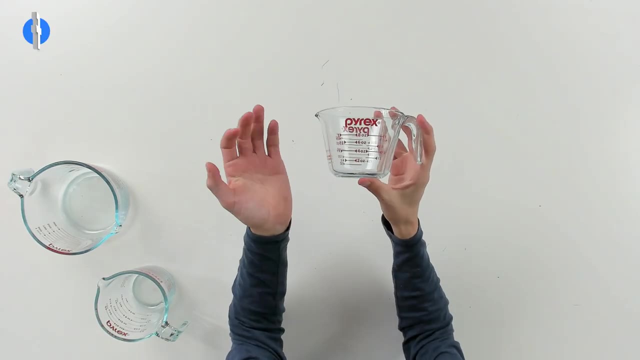 glass measuring cups. We have a one cup, a two cup and a four cup option. Let's go ahead. let's look at those in more detail. First up, we got the one cup right here, so check it out. Two, four, six, eight ounces We can look at from the other side. we have our metric units. 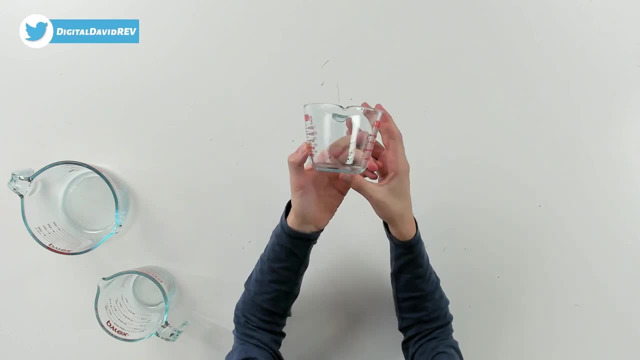 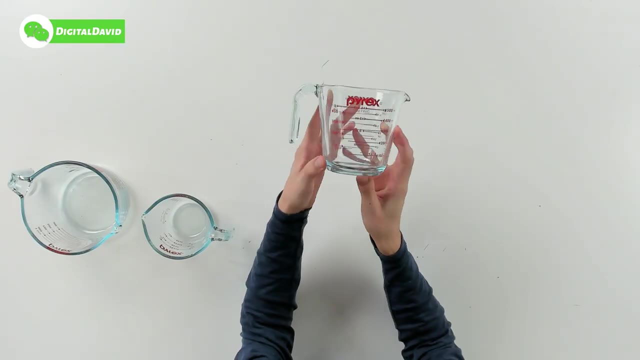 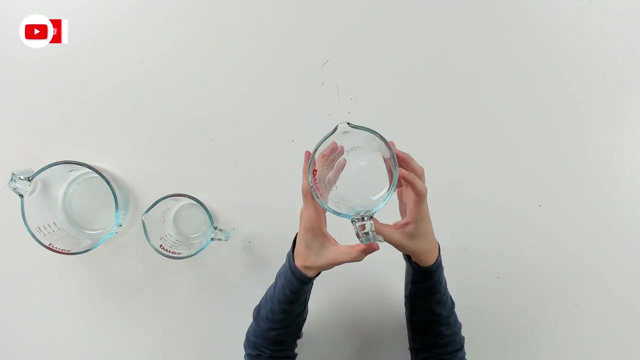 and milliliters Made in the USA for microwave use, not for stovetop. This is also oven safe. Now we can look at the two cup version. So obviously twice the capacity. Everything looks great. 16 ounces And lastly we have the four cup. 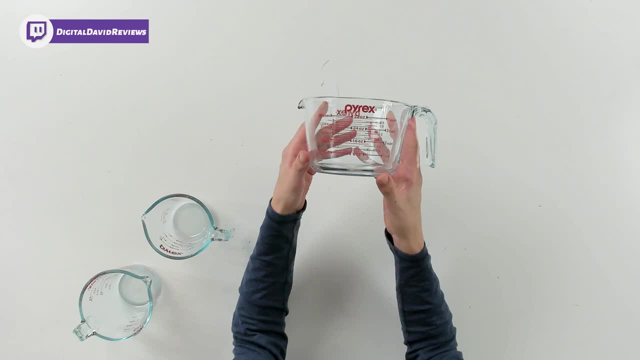 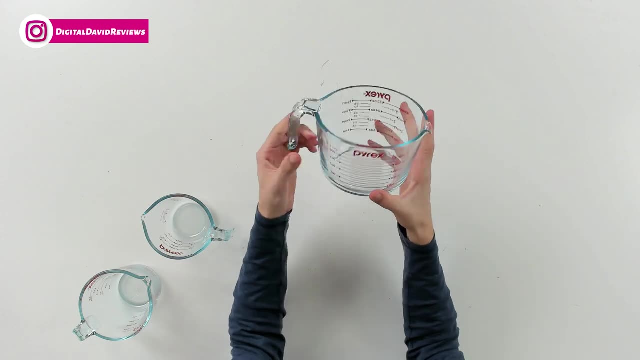 version right here, So check that out. 8,, 16,, 24, and 32 ounces, Cups and quarts. Then we have our liter and milliliters on the other side right there. Great construction, Everything looks great. 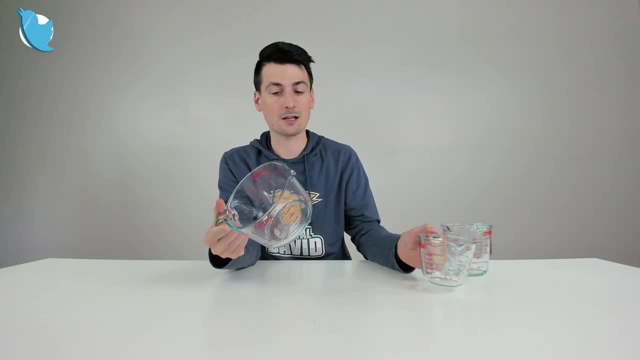 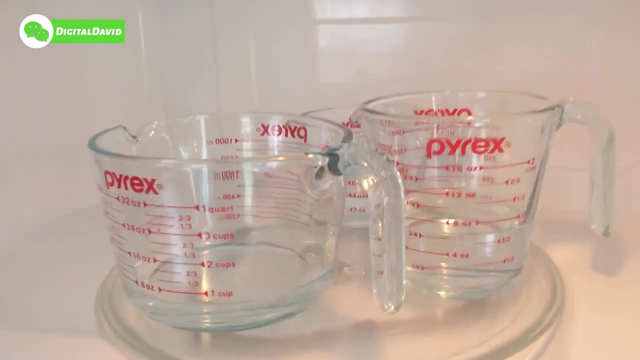 Nothing's cracked, damaged or anything along those lines. They have a good weight to them, as you would expect, since they are glass. Now let's go ahead and let's try them out. So first up, you can see we have all three of the glasses in the microwave. So let's go ahead. let's start it for. 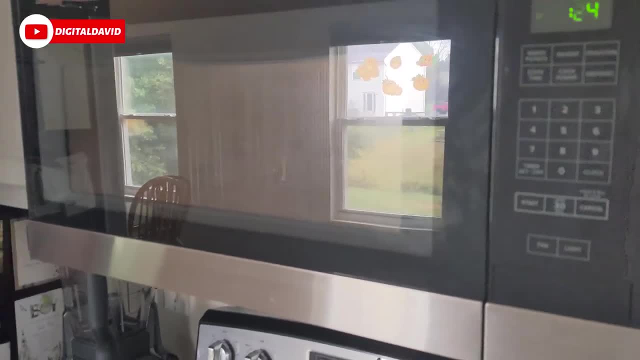 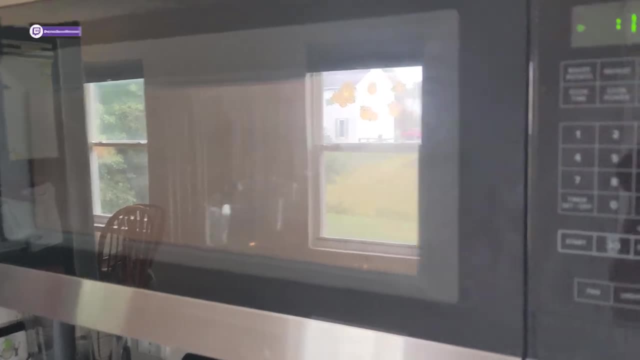 you. You can see the microwave's operating just fine- No issues with them being in the microwave. So far, so good, As you would expect, since these are microwave safe. Now we can go ahead, we can open it up and you can see no issues at all. Now you can see, I have